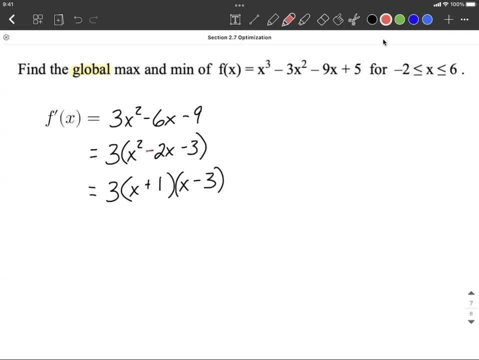 minus 3, we'll end up with this negative 2 in the middle. All right, this is going to point us towards having critical numbers or critical values at. for this x, that would be at x, equals negative 1.. And for this x, that's going to be at x, equals positive 3.. 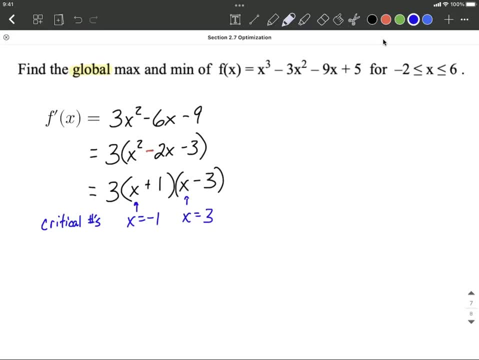 So you may be saying, okay, well, that'll make the derivative equal zero, So we have a possibility of a maximum or minimum there. Those could be local, they could be global, we're not really sure. From here, it actually is pretty. 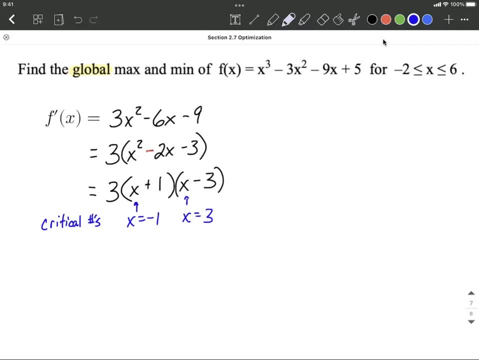 easy the rest of our steps. All you have to do to finish this problem is you want to evaluate back into the original function negative 1.. So negative 1 cubed minus 3 times negative, 1 squared minus 9 times negative, 1 plus 5.. And I think after you work this all the way down, you get. 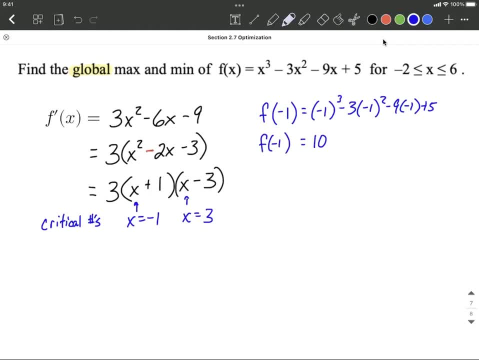 10.. So f of negative 1 equals 10.. We also want to do the same. We're going to do the same thing with 3.. So f of 3, back into the original And, after a little bit of work, maybe use your calculator to help you out. 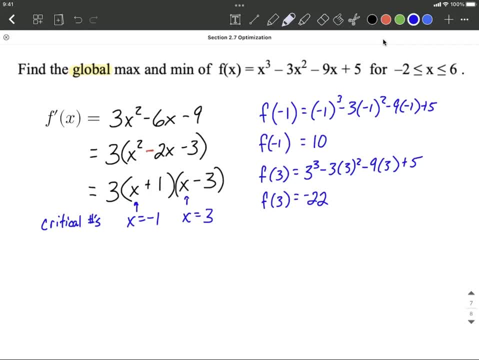 we should get negative 22.. So I know at this point a lot of students stop and they say: okay, 10 is big, negative 22 is small. All right, it's much smaller than 10.. So we must have a global. 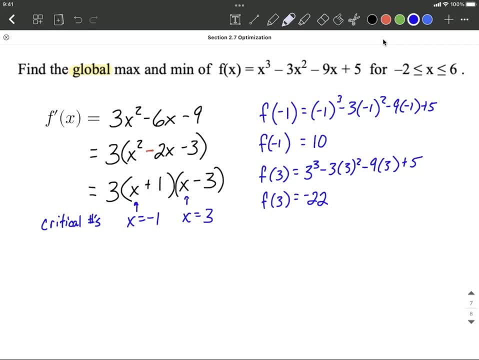 maximum at negative 1 and a global minimum, I should say at the y value: maximum at 10, minimum at negative 22.. However, where students forget to look, is they narrow down which x values we're looking at. All right, we're only looking. 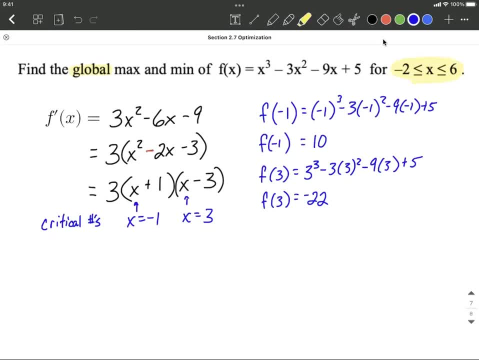 between negative 2 and positive 6.. So, sure enough, negative 1 and positive 3 both fit in that range of values. for x, However, there's a possibility that we could have an endpoint at negative 2 or at 6. that's actually bigger or smaller than these. 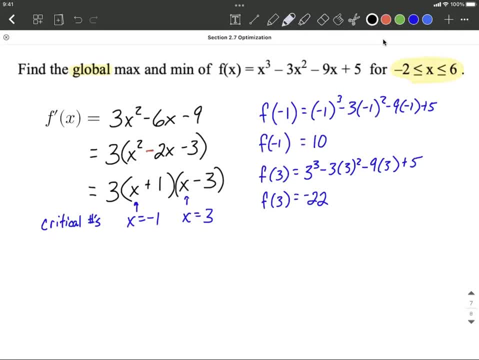 So what we want to do is also go back and evaluate our original function at negative 2 and at positive 6.. Okay, so negative 2. as we replace each one of the x's again in our original function And work this all the way down, we get f of negative, 2 works out to be 3, and f of 6,.